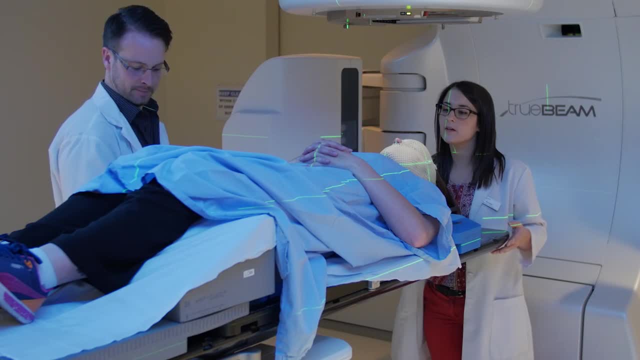 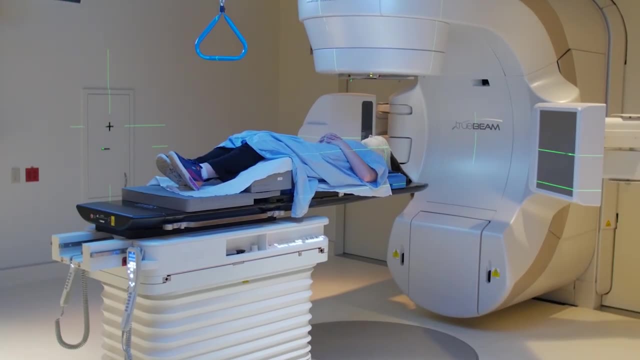 So once we're happy with the patient's positioning, we will let them know that we are leaving the room. and just to hold still Now the radiation therapy staff. as much as they would like to be in the room with the patient during the treatment, we can't, So we have. 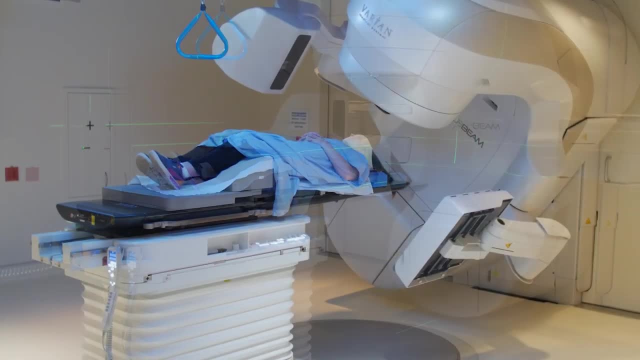 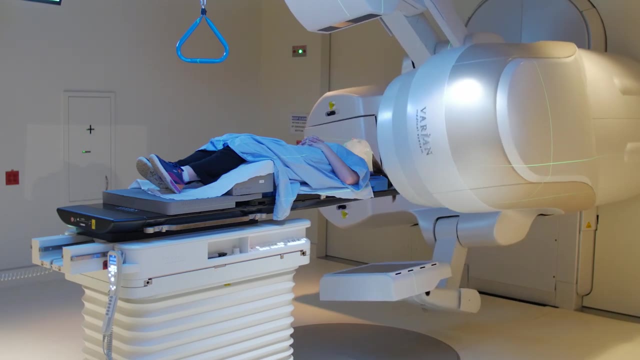 to stay outside. The machine rotates around them, but they will not be touched by the machine When the radiation starts. they cannot see it, smell it, taste it, nothing. They may hear a bit of a buzz in the background and they also hear a little bit of a clunk, and 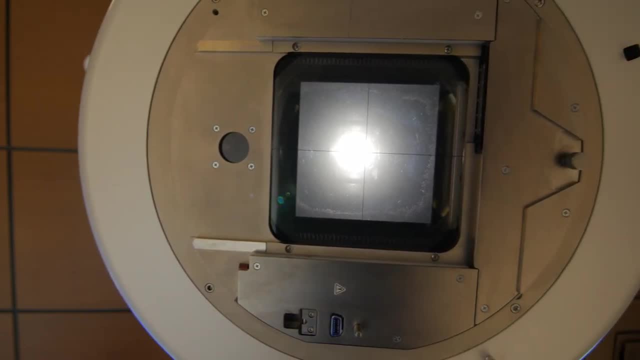 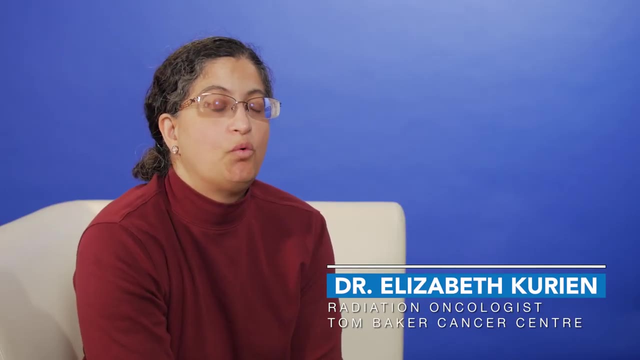 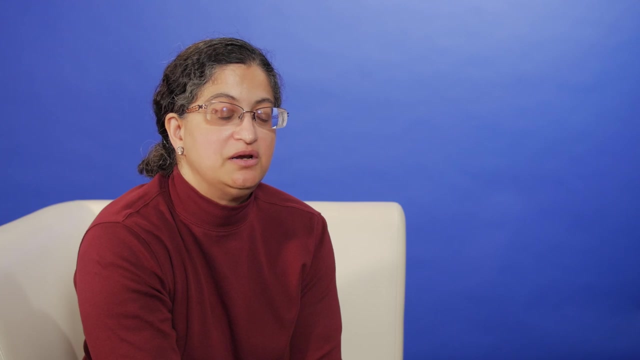 that will acknowledge that the machine has started When you're lying on the bed. the machine does move around. The radiation can be delivered from one position, or it may be delivered as the machine moves around you, or you may find that the machine moves to a different position. delivers some. 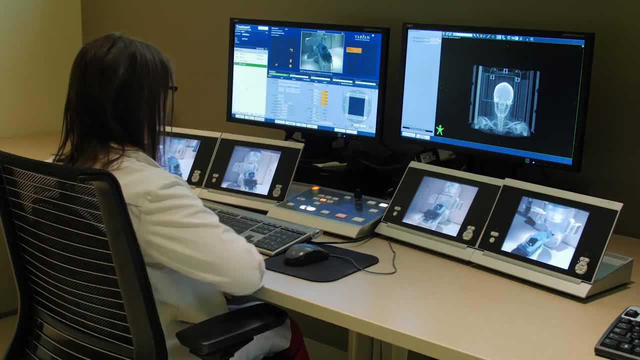 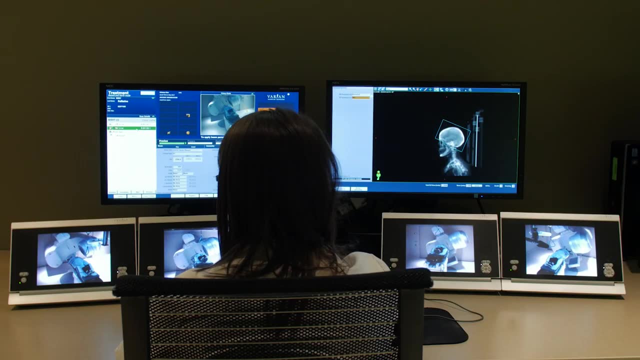 radiation, moves to another position, delivers some radiation and like that. So it's different for different people. Despite you being left alone in the room, you are being monitored from the outside. Your therapist can hear you from the outside of the room and they 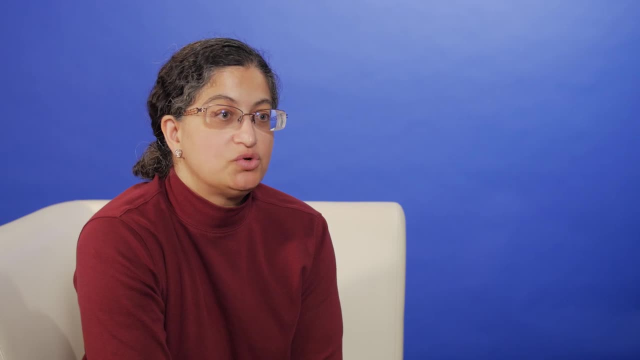 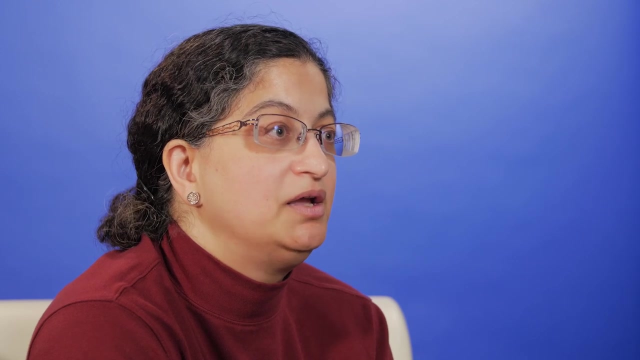 can see you from the outside of the room and they will give you instructions so that if you are uncomfortable or afraid, you can always signal them, either by voice or as they indicate to you, so that they can stop the treatment. come in check. what's bothering? 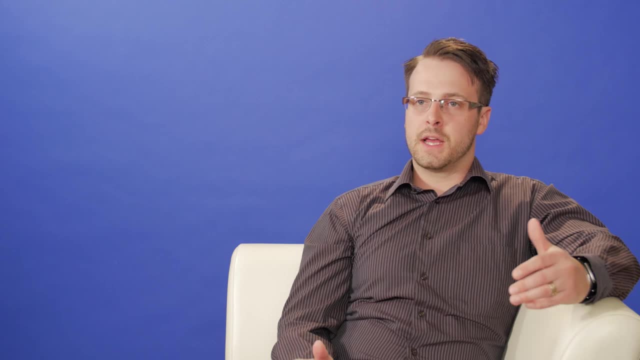 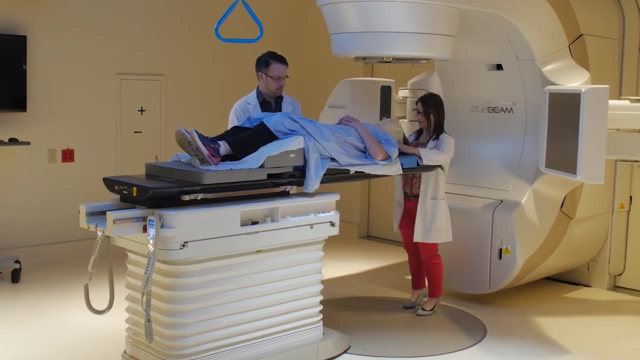 you, They can make sure things are good. So once the treatment has completed, the radiation staff will come into the room, bring the patient back down to the ground and give them a little bit further education on how to treat radiation. The radiation staff will come into the room, bring the patient back down to the ground and give them a little bit further education on how to treat radiation. 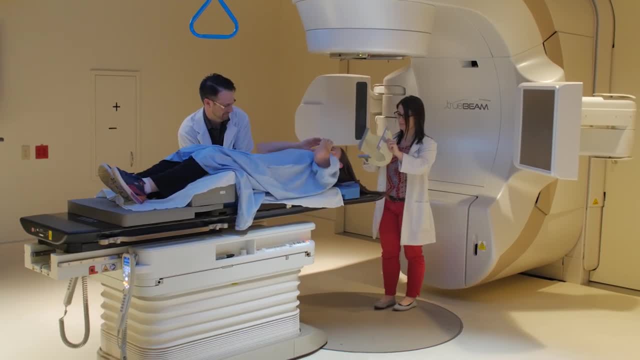 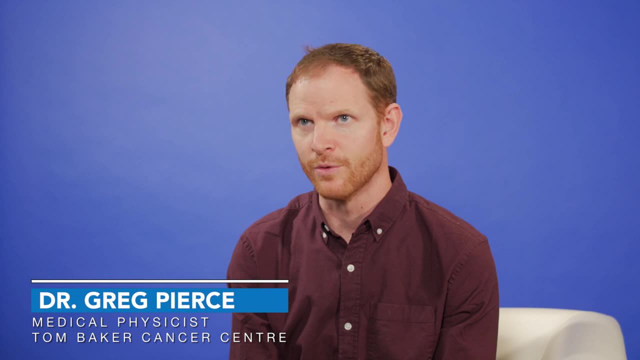 And what kind of radiation does that require, given the comfort in that room and how it can affect their Carlton Hospital? Sir Robert Ines In적, I know that patients often wonder why they receive different doses and fractionations, Different tumor cells in different locations in the. 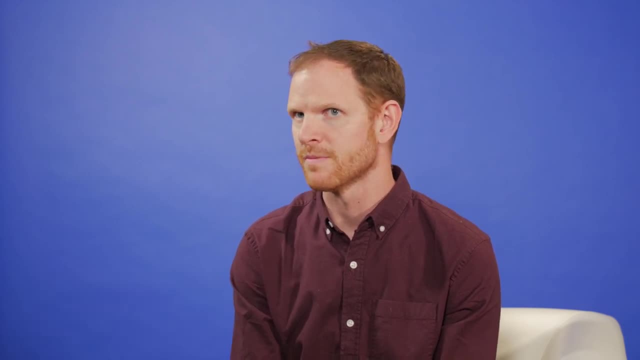 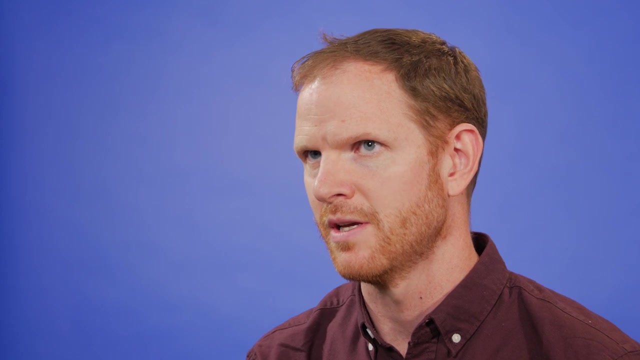 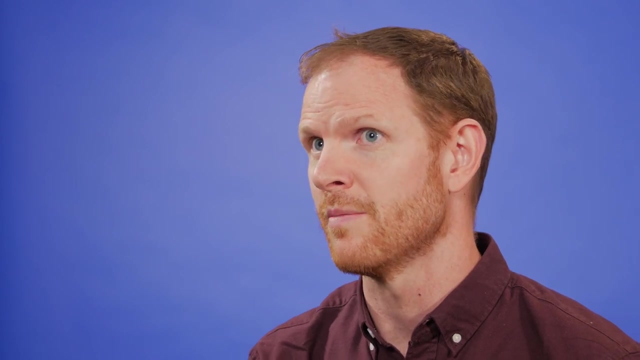 body respond differently to the radiation and as well your body responds differently to amounts of radiation and we, basically we cater the amount of dose specifically to different sites in the body And some also some patients receive chemotherapy in conjunction with this and some people have had surgery beforehand. So different amounts of radiation. is very, is tailored very specifically to different types of cancer. In hindsight it seems like it went faster than it did, probably, And then each one got just a little bit easier. The treatments themselves, the appointments themselves got easier. I knew what to expect.